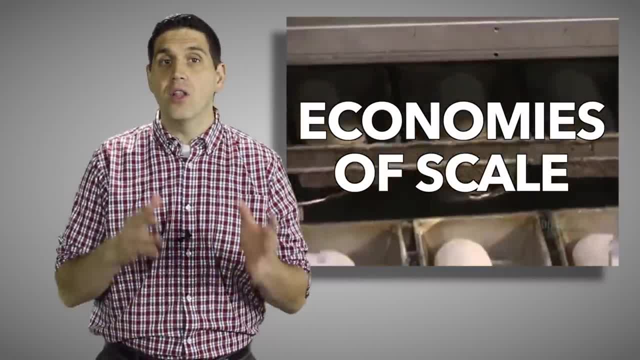 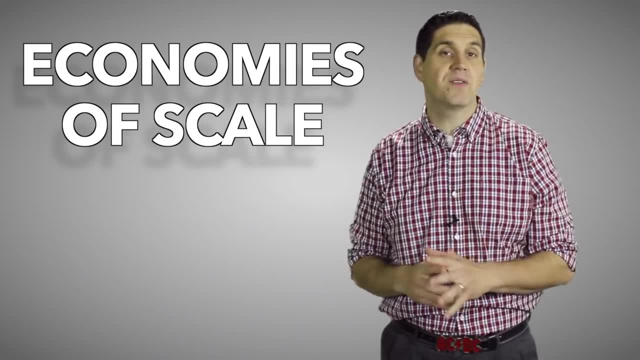 It's way lower, And that's the idea of economies of scale. The long run average costs fall as more output is produced. Economies of scale is the idea that getting bigger is cheaper. It happens because of increasing returns to scale and other cost-saving measures. Companies that are producing 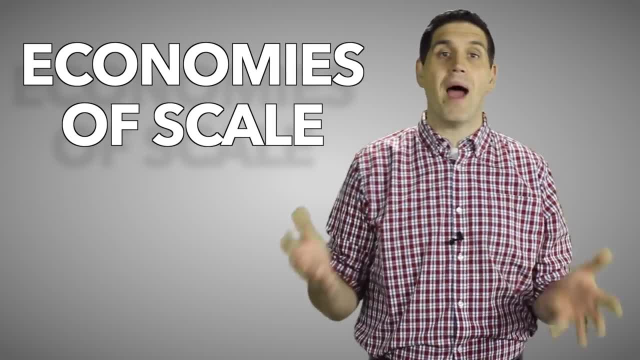 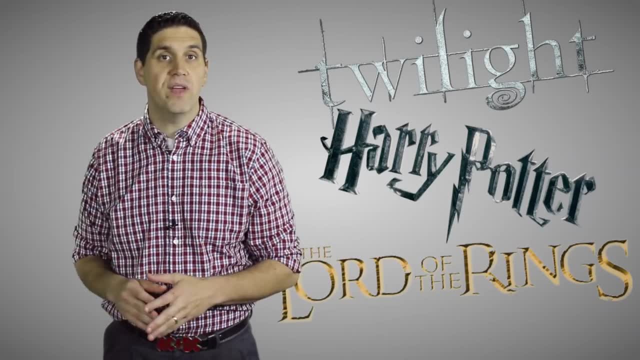 at a larger scale, can afford super productive machines and also buy resources in bulk. Again, the total cost might be a lot higher, but the average cost is lower. And that brings us back to those movies. Several of the Twilight and Harry Potter movies and all the Lord of the Rings movies were shot at the same time. The total cost: 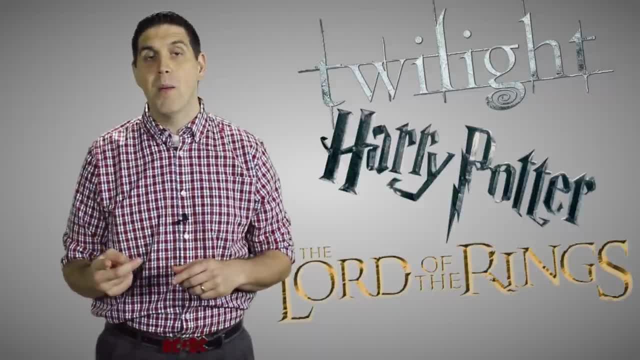 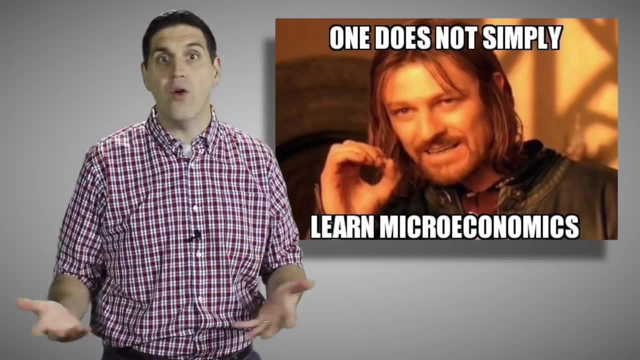 of producing three movies is a lot more expensive than just producing one, But if you produce them all at the same time, the average cost is going to fall. When they made the Lord of the Rings, they didn't have to ship their cast and crew to New Zealand over and over and over again. 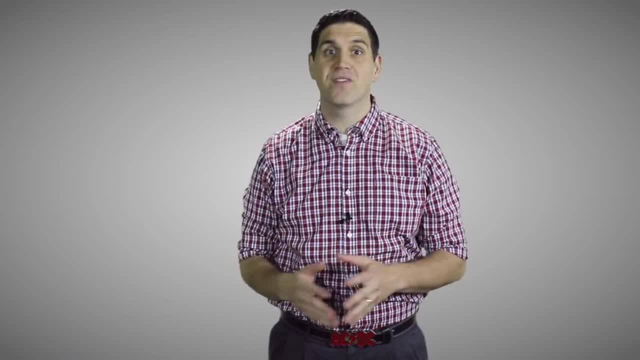 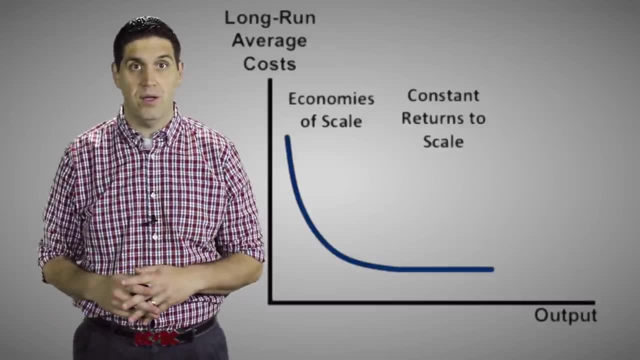 So producing multiple movies all at once meant that they had economies of scale, But often costs don't keep falling and falling in the long run. Like production, they often level off And this is called constant returns to scale. So when you're producing bread, there's just no way to get. 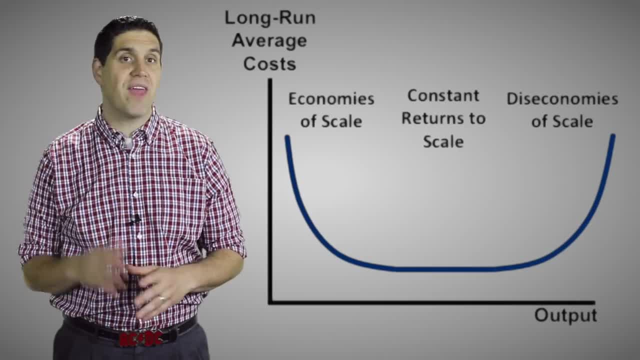 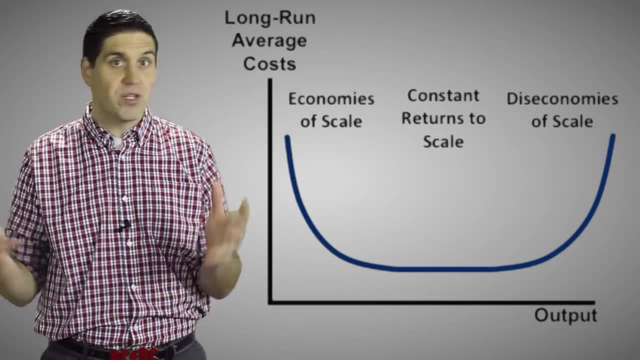 your costs below a certain amount per loaf And eventually it's possible for the average cost to start going up as more is produced, And that's called diseconomies of scale. In that situation, a company becomes so big and is producing so much that they have to hire extra managers. 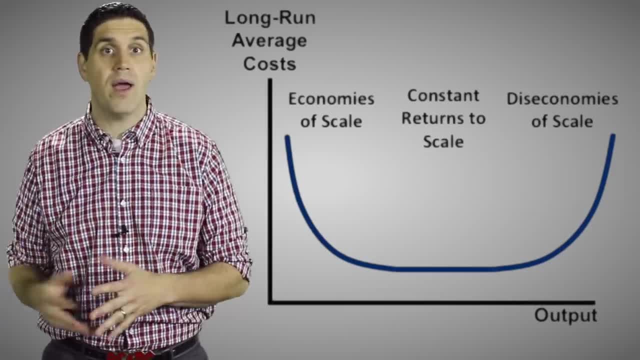 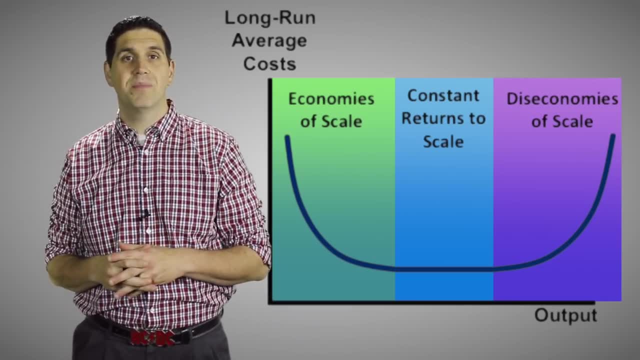 they have to add a cafeteria to their factory, so their average costs start going up. Now you might be thinking that a firm wants to produce where they have the lowest long-run average cost. but it's not that simple. The amount of firms should produce, they're going to have to. produce doesn't just look at costs. it also looks at consumer demand. I mean, think of your local pizza restaurant. The goal isn't to minimize their costs. make as much pizza as possible. Their goal is to maximize profit. Think about it: they could have advanced pizza making robots that do. 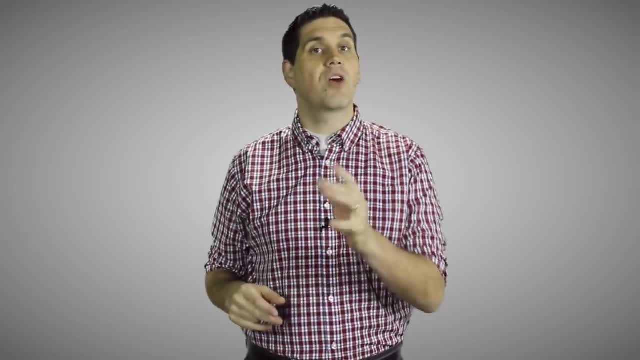 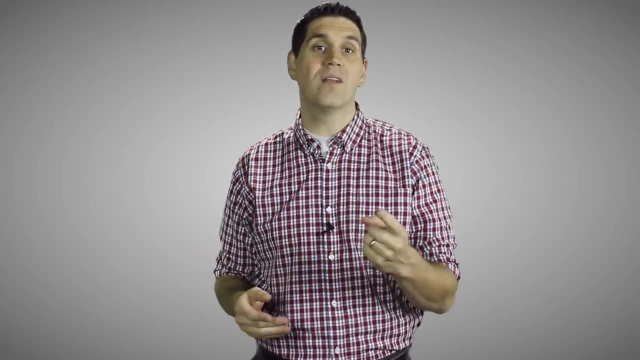 all the work, but they don't sell enough pizza to make it worth it. The point is, concepts like economies of scale are ideas that help producers make decisions. They don't tell producers exactly how much to make, because in real life, one size doesn't fit all. Thanks for watching until next. 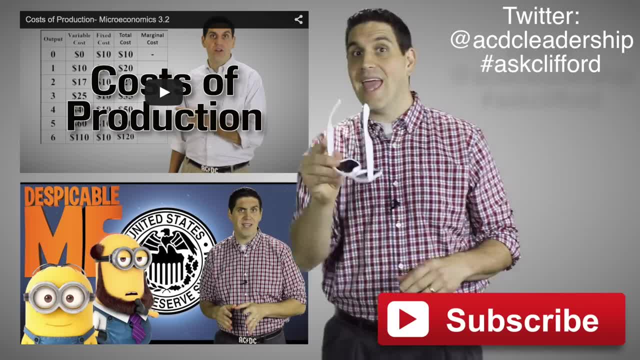 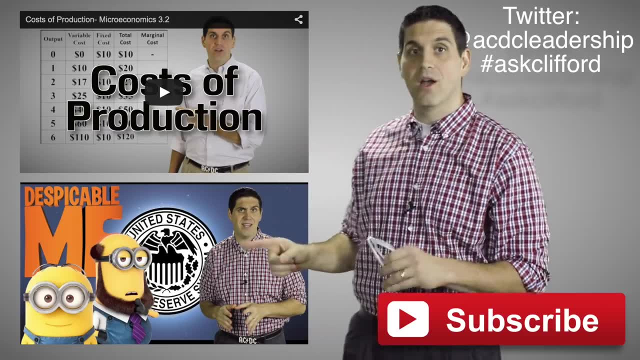 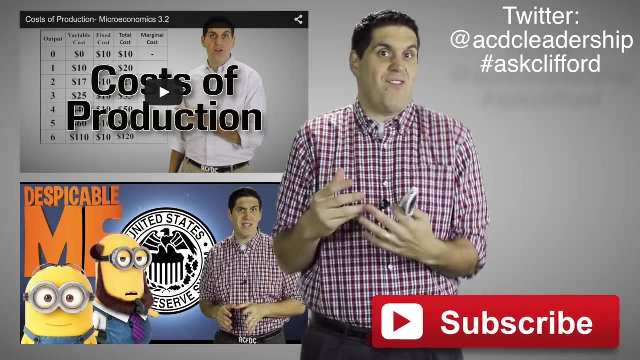 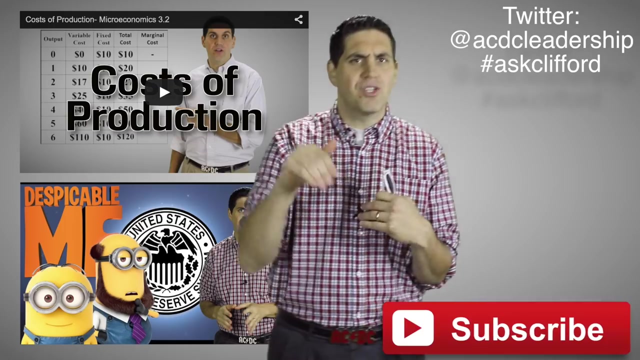 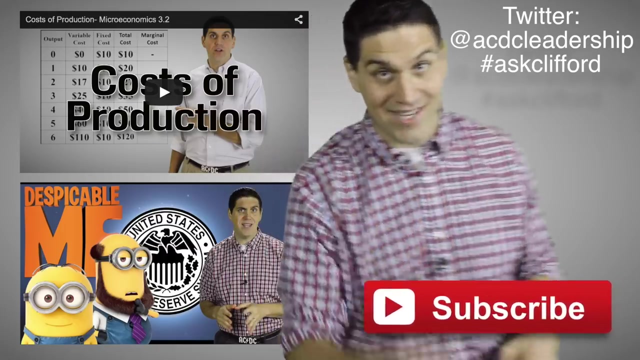 time. Please like and leave a comment. If you want to learn more about the cost of production, click right here. If you want to learn more about economics by looking at movies, click right here. Also, please make sure to subscribe. Subscribing tells me you like the channel, you like the videos and you want to see more of them. okay, Whatever, you don't have to, but it'd be cool, You know? I mean, I know you want to. You want to subscribe, man? Seriously, go ahead and click on it. Don't look at me, just subscribe. You can do it. You're doing it right now, aren't you? Yes, awesome. Hey, I knew I could trust you, man. Hey, thanks for watching, Until next time.